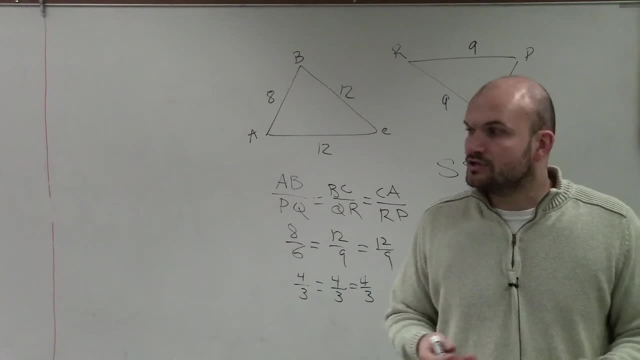 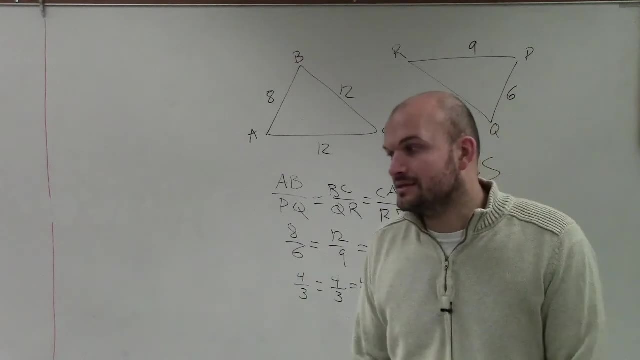 If you have three sides that are proportional for our two triangles, then you can say that they are similar, Right Meaning they have the same size, but not necessarily the same shape. OK, So that proves similarity, because 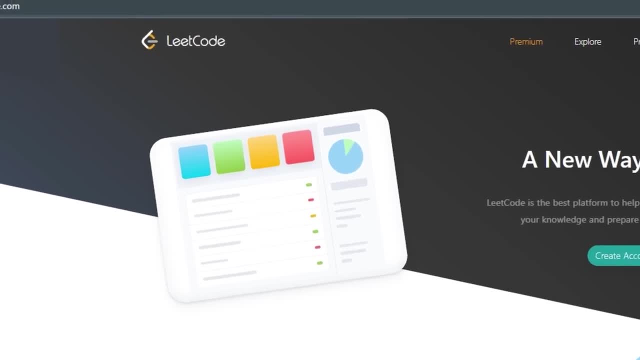 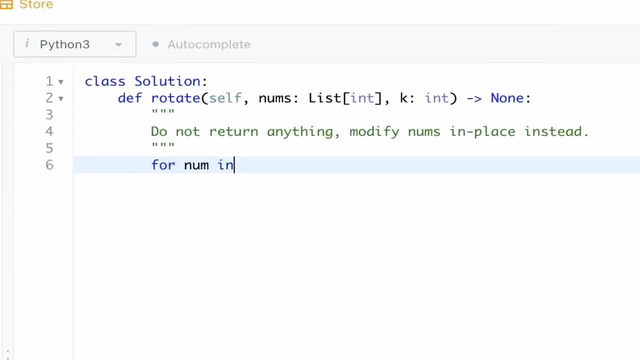 Coding interviews are very easy. That's what I thought when I went to Leetcode and attempted this rotate array as my very first problem. After spending six hours on it, I had not written a single line of code. I was extremely frustrated and went to the discussion section. 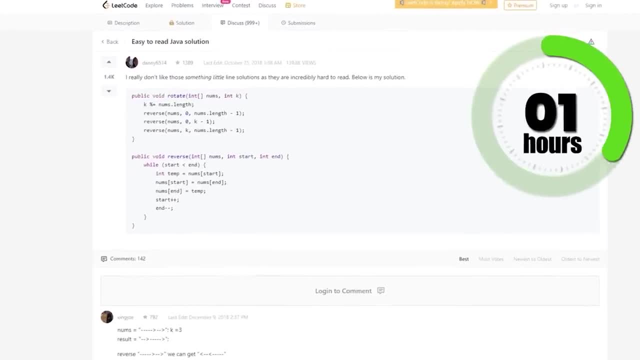 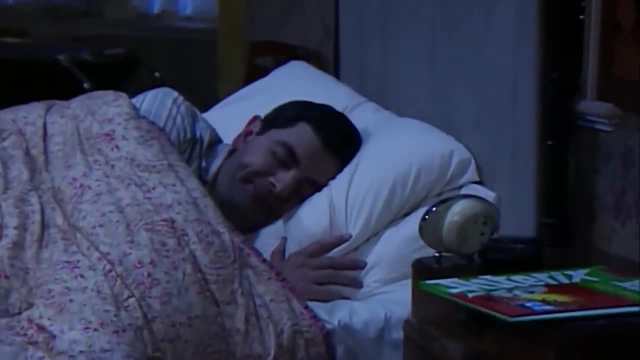 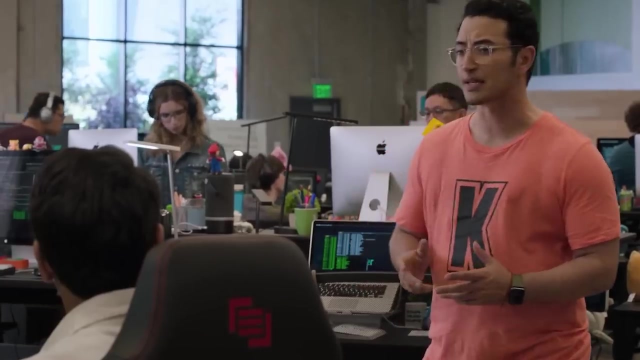 to read the most upvoted solution. Another two hours passed and I could not even figure out why this solution works. At this point, my frustration had transformed into disappointment. I somehow managed to put myself to sleep that night. In the next morning I went to a friend and asked him to solve the exact same question. 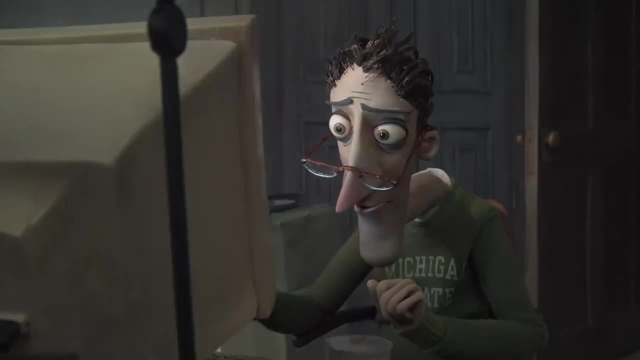 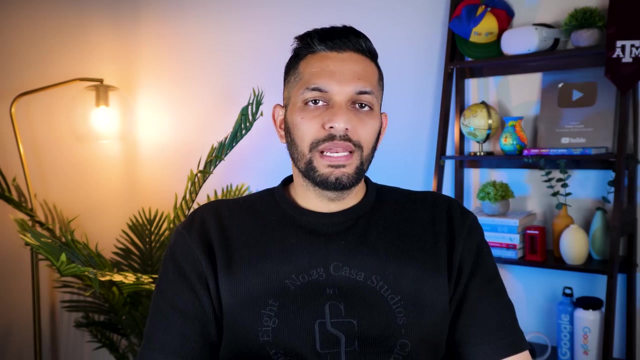 And that's when I learned something interesting about the human behavior: If you cannot solve a problem, you feel sad, But if your friend solves the exact same problem in under 15 minutes, you are heartbroken. After facing many hurdles like that, I managed to solve. 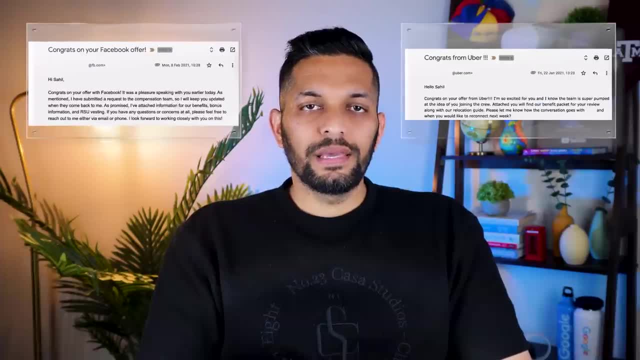 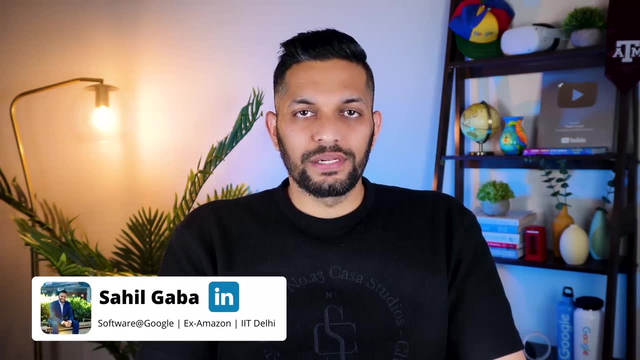 more than 500 problems on Leetcode, And along the way, I collected many amazing job offers. Today, I'm going to share everything that I've learned in the process. At the end of the video, I'll also answer a very important question, And that is: 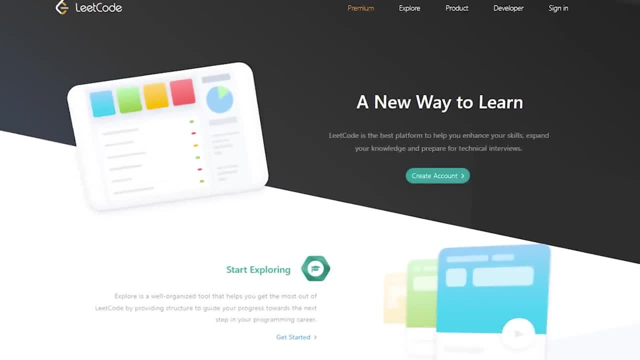 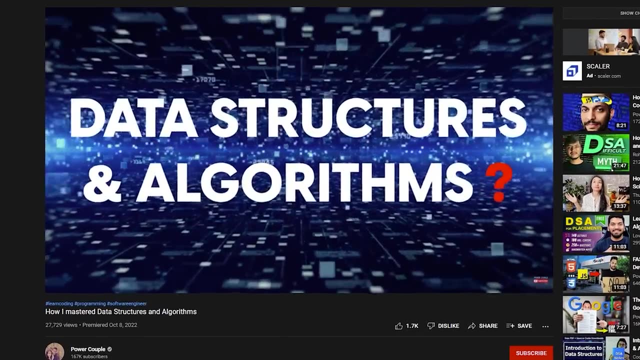 How do you solve problems in Leetcode? How to know if you're ready for interviews at big tech companies? Before you can even start on Leetcode, you need to have a good understanding of data structures and algorithms. I've already covered this topic in my last video, which I'll link. 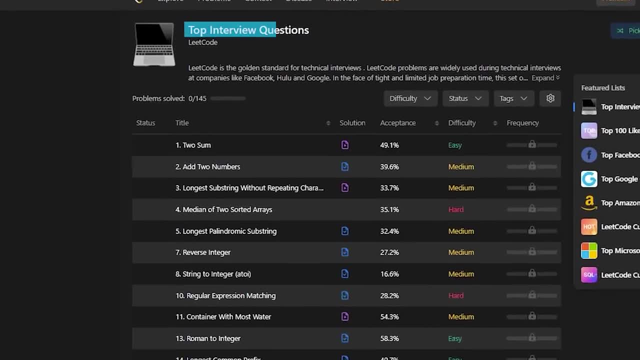 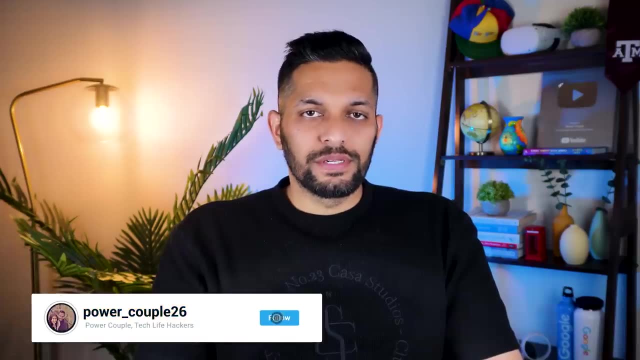 at the end. Once I finished the basics of DSA, I went to the top interview questions on Leetcode. There are exactly 150 problems in there and all of them are very important. I recommend that if you're solving a problem which is outside, these 150 problems make.